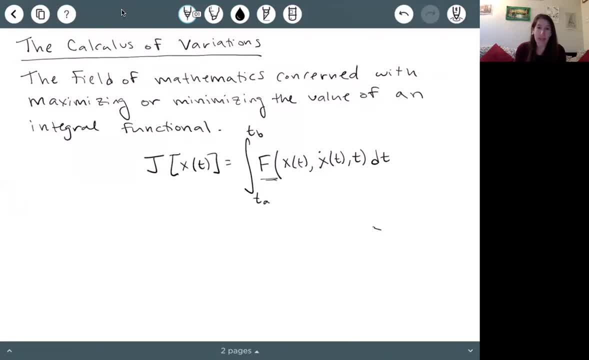 where here f is some function of x, x, dot and t. We're trying to find the value or the function x that extremizes j, All right. so this is a fairly complicated problem that we're trying to answer here And I'm not going to prove for you. I'm not going to prove for you, I'm not going to prove for. 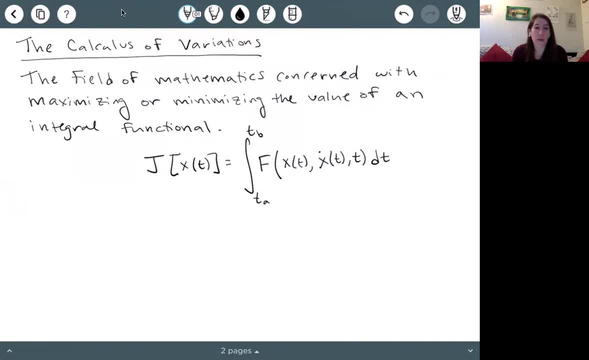 you what the answer, how to do this. but I'll show you what's known as the Euler-Lagrange equation, which is a solution to this problem of how to find the function x of t which extremizes j. But before I do that, I just wanted to sort of give you an idea of where calculus of variations 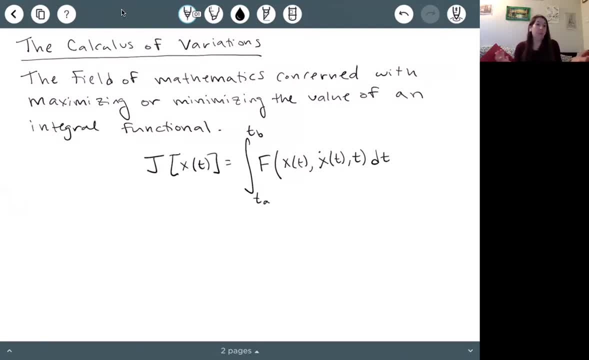 is important in physics because you could just look at this as simply a math problem. You're trying to do this extremizing math, But it turns out to be quite commonplace in physics, where it turns out that nature likes the extremum of things. So the solution to many physics problems is that you need to. 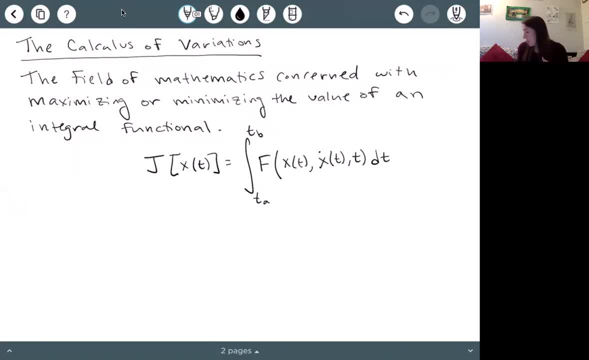 extremize some integral, functional. So examples where it comes up. so maybe you've seen in optics Fermat's principle which tells us that light, the power of light, is the power of light. So the path that a ray of light will take is the path of shortest time. Another place that it comes up. 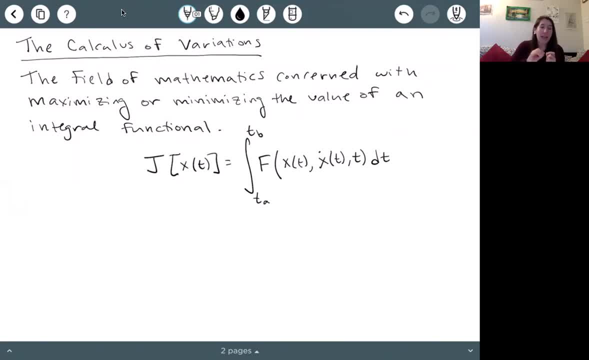 is in general relativity. So the paths that particles follow in general relativity extremize what's known as the proper time along that path And then in classical mechanics. so for us it'll be important because in Lagrangian's formulation of classical mechanics 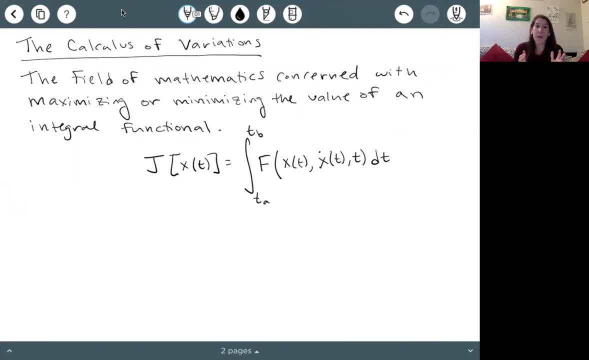 it turns out that the trajectories of particles, or trajectories really of systems, are given by the extremum of what's known as the action of that system, And we'll see more about that in the future videos. So the general solution to this is given by what's known as the Euler-Lagrange equation. 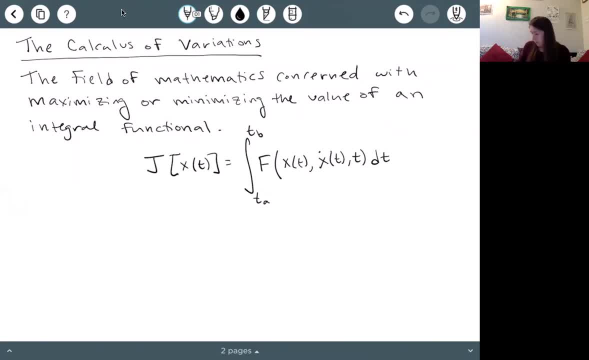 We can put in 0 and if you put a pointer on a board that says x, B-x, b-and you can transmit it to me with this epaged pen straight to this column of Time. So if you take the time, derivative of the partial derivative of this function, f with respect to x dot. 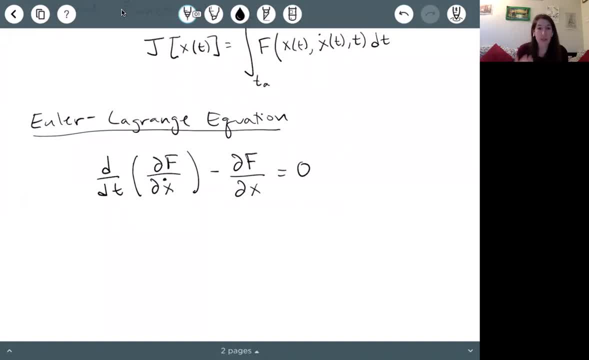 and then subtract the partial derivative of f with respect to x and set that equal to zero, and then echiz parentheses cease at the capital. Nice equation, ultimately, that we can solve for x, then that function x, subject to whatever boundary conditions we might have, will be an extremum of j, So j or a will be the extremum, So something. 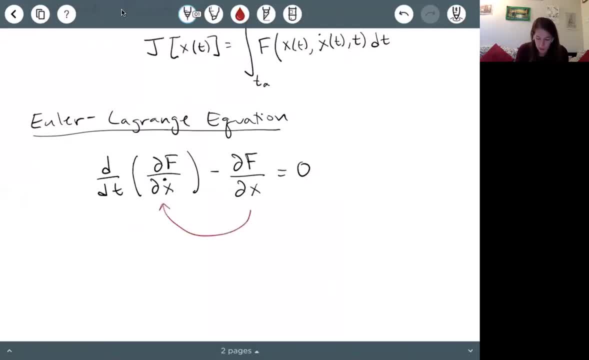 very important that I want to point out here is in these partial derivatives you're going to treat x and x dot as though they are independent variables, which might sound strange. but so when you take the partial derivative and you hold everything fixed in this first, 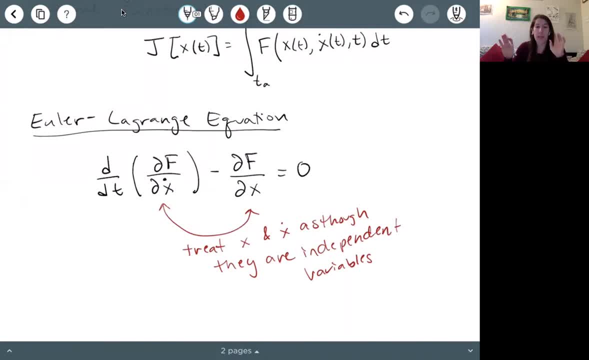 guy, you hold x fixed and take the derivative with respect to x dot. and then, in the second term, you hold x dot fixed and take the derivative with respect to x. so you're treating x and x dot as though they are independent variables of our function f. And then the solution to this. 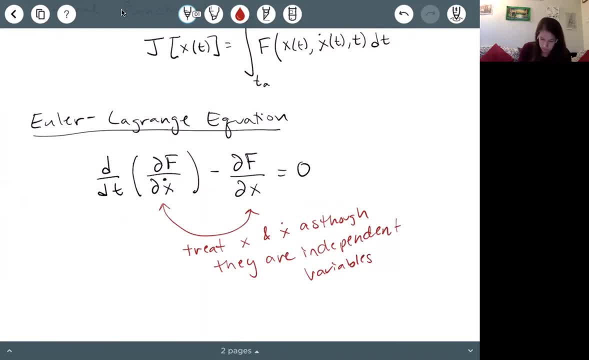 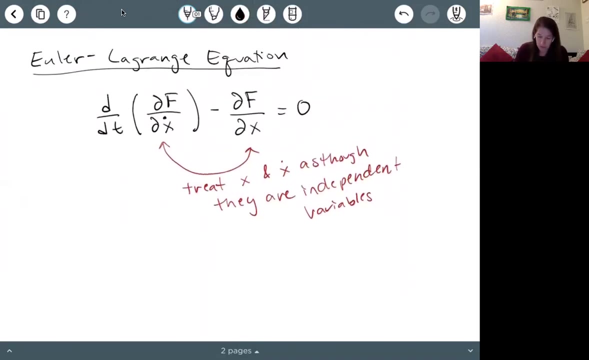 again will extremize the function j. So the last thing I wanted to do in this video is just give you a little bit of a summary of what we're going to do in this video. I'll give you an example of the types of problems that we use the Euler-Lagrange equation for 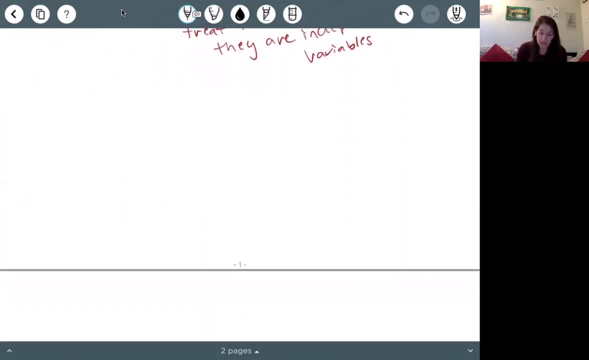 and specifically, I'll give you an example of geodesics in space. So these are spatial geodesics which are simply the paths of shortest distance between two points. So, for instance, in flat space, if we have some point A and B and we want to find the path of shortest distance between two points, 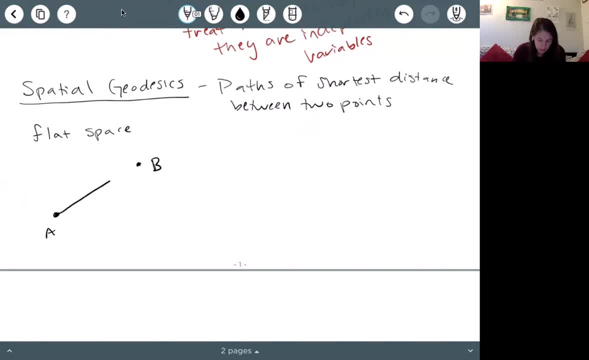 probably most of us already know the answer to this question, which is that the path of shortest distance between two points is the path of shortest distance between two points, But it's just going to be a straight line, So this would be the geodesic. 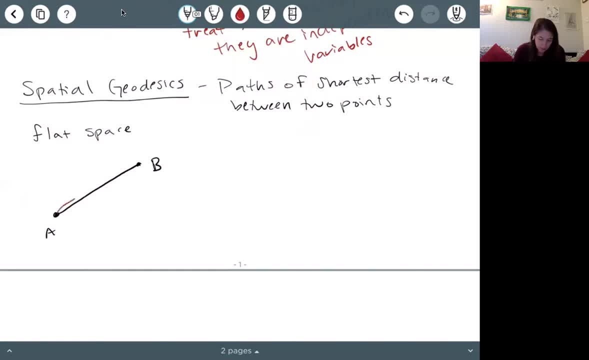 And you can imagine if we took any slight variation from that short line, any type of variation we might want. right, any of these paths are going to be longer than the straight line distance, So we would say this black line is the geodesic. 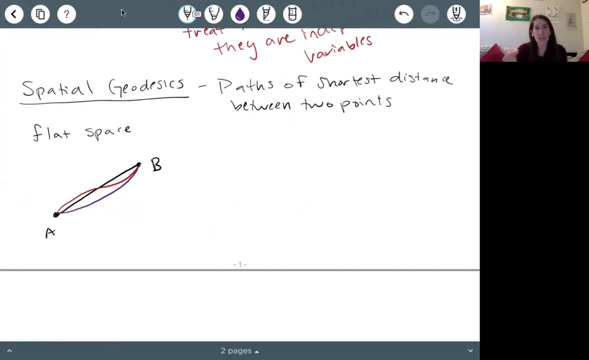 subject to the boundary conditions that it is a geodesic that starts at point A and ends at point B. Now in flat space, this problem again, we've all seen it. but maybe we're in flat space and maybe there was some obstacle in the middle. 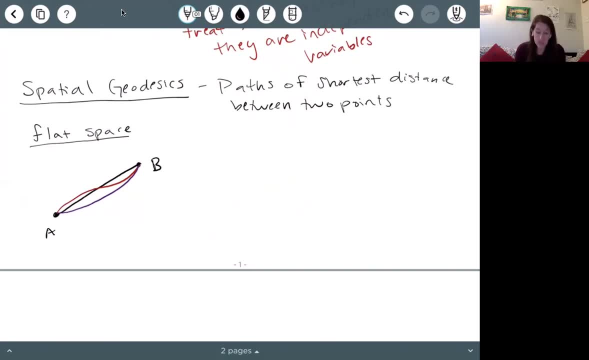 and then the path has to go around that obstacle. So then that would be a slightly less trivial problem. Or maybe we were on the surface of a sphere and we're trying to find the shortest distance between two points, Point A and point B, on the surface of a sphere. 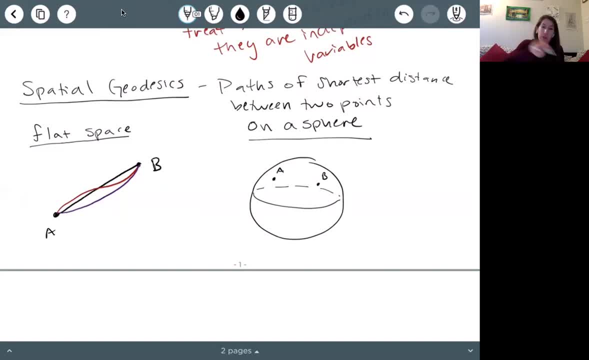 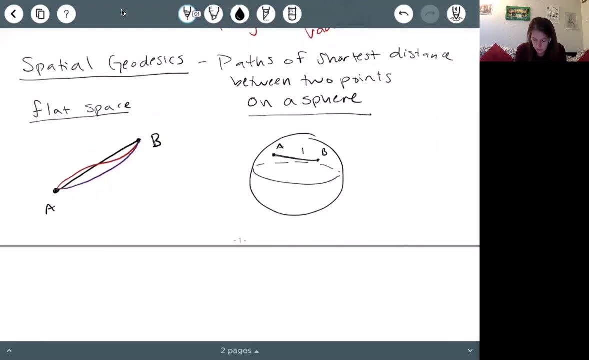 which, now, this is a less obvious problem if you're constraining your path to be on the surface. Now, it turns out that great spheres are great circles on the surface of the sphere, which is to say, circles that go all the way around. 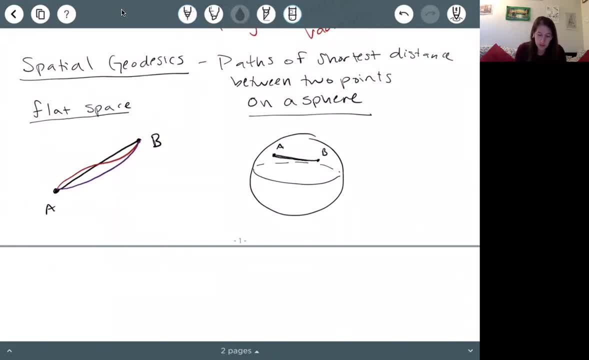 So parts of these great circles are the geodesics? Oh, okay, But this to me would not be totally obvious, Like I wouldn't know, like do you just try to you know you could imagine drawing all sorts of different paths between these two points.